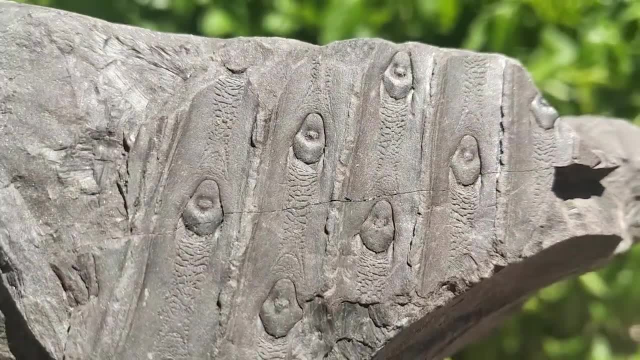 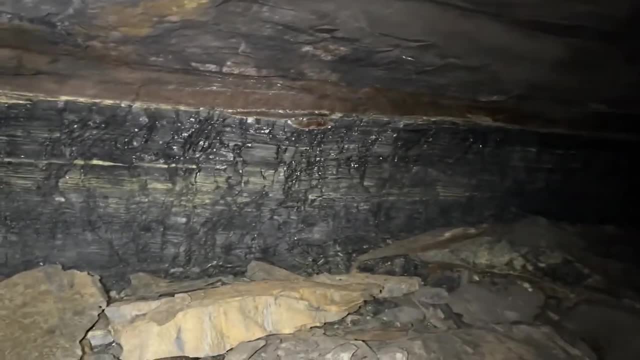 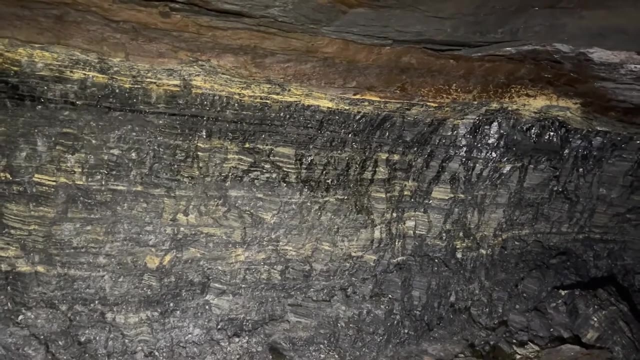 was one of the most leading components of the swamp forest, aged off 300 million years ago, An age that belongs to a famous geological period named according. to all core deposits we found from this glooming and unknown time, It's Carboniferous. So what type of plant was it? 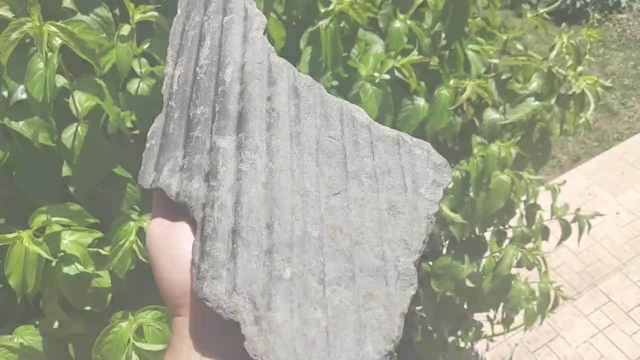 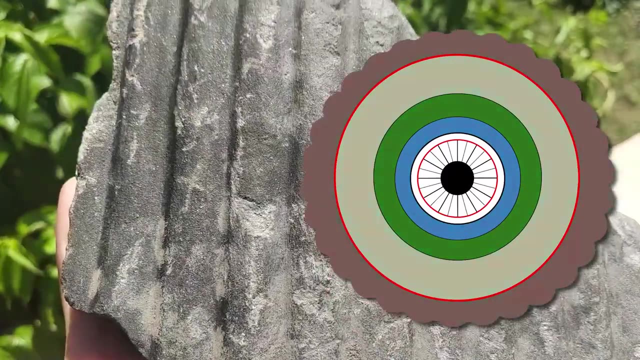 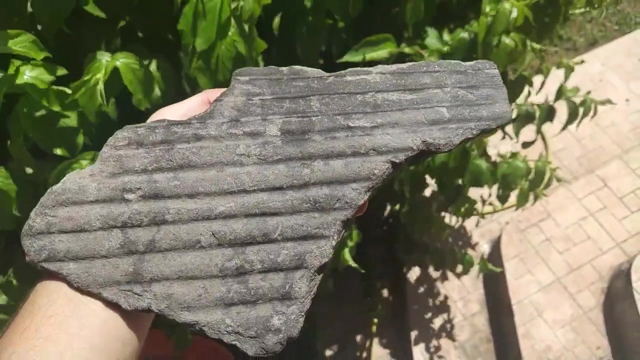 And what did it look like? This sample that you can see here is, in fact, a part of the outer cortex in a sigillian stem. More precisely, it's identified as an example of a huge fossilized bark. Paleobotanists that seen this fossil plant remains called it Syrangodendron, a name which 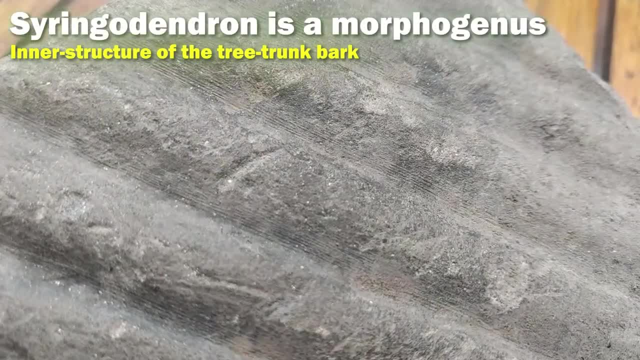 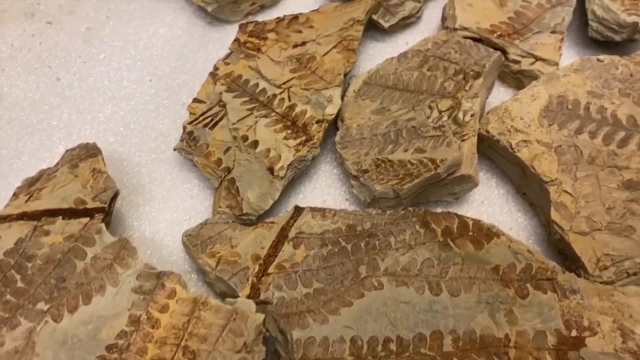 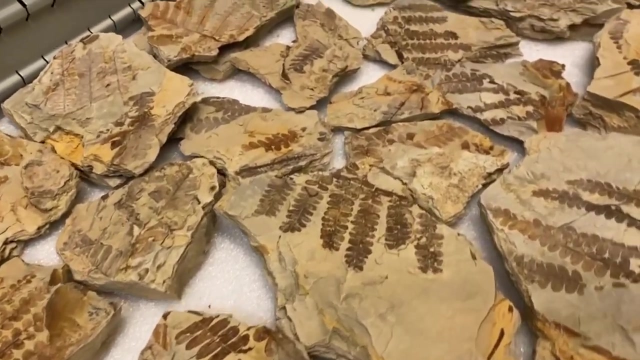 is considered as a morphogenesis. Indeed, even if there is an abundant amount of fossil remains for plants, we have rarely found connection between several different plants' organs. So most of the time, fossilized plant organs are scattered and paleobotanists must give. 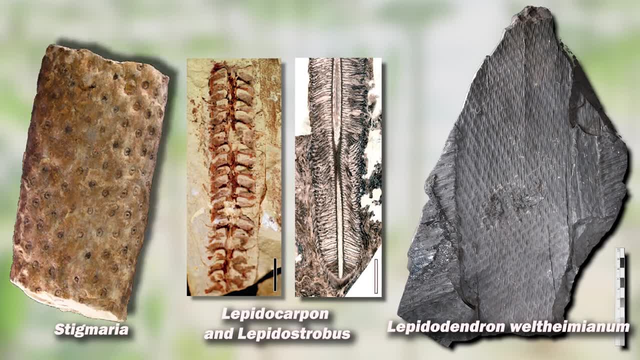 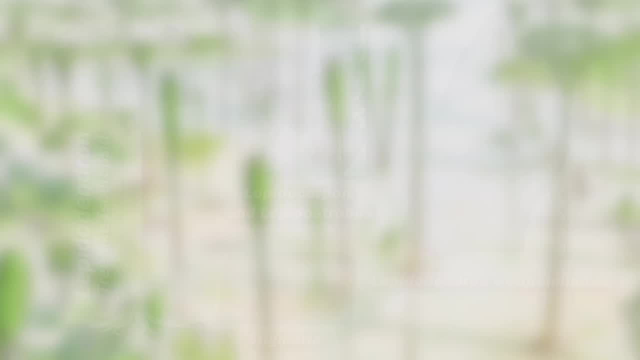 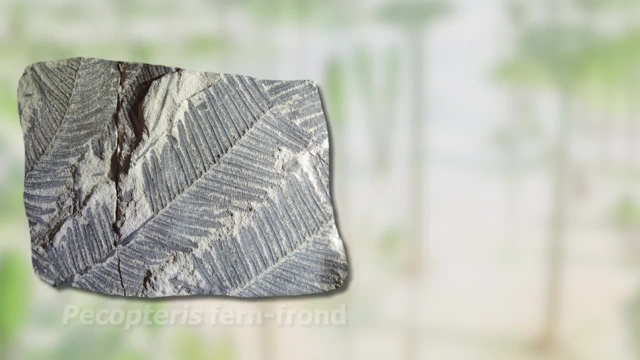 to each one of them a name, which would be a morphogenesis that depicts a specific plant organ on an extinct plant species. For example, Pecabteris, one of the most famous fossil ferns, is described as the leaf part of an arborescent lamarischal. 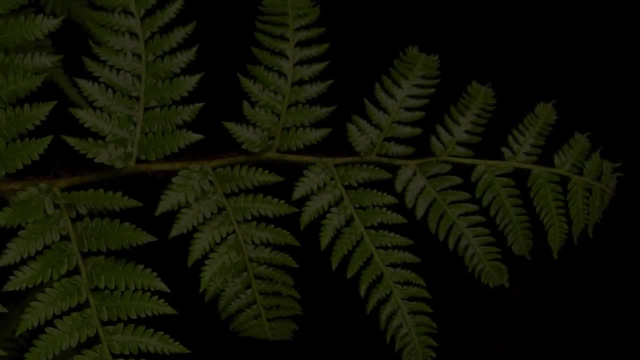 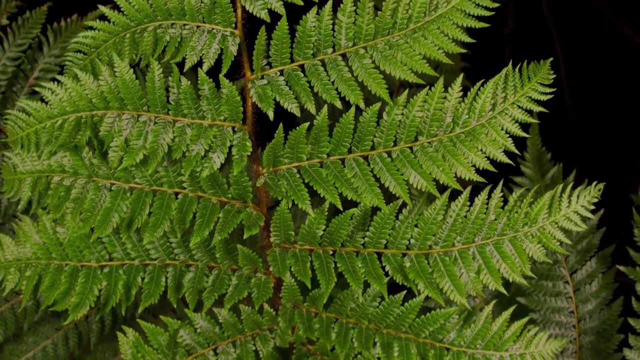 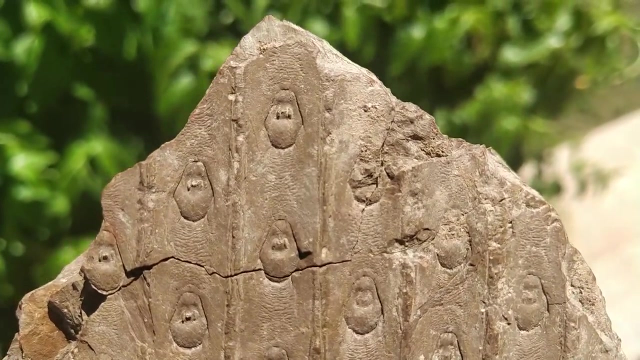 A tree fern called Saracen- Thus, Pecabteris is a morphogenesis- a fern frond which belongs to an extant tree fern, Psirrhonius. Go back to our tree trunk bark. Sigillia is a tree-like club mosses featured by these leaf scars, which contains leaf cushions. 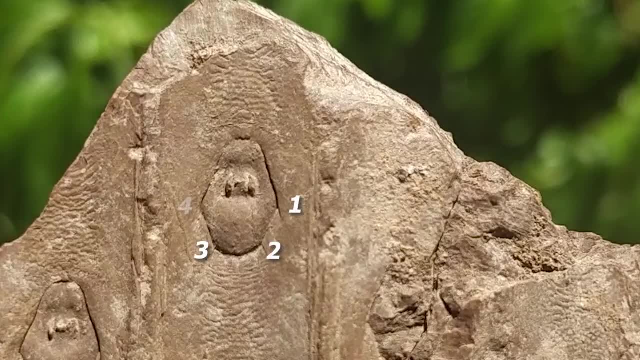 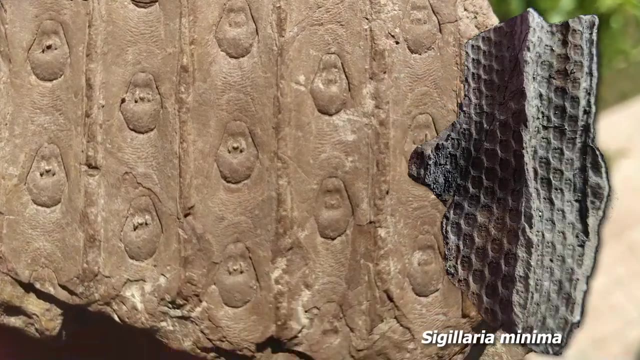 Sigillia leaf scars are easily recognizable by their hexagonal shape, with a legular pit at the top and two characteristic leaves. They are also known for their shape. These hexagonal leaf scars are organized in a linearized structure which gives them a shape of a scale tree, just like its close relative Lepidodendron. 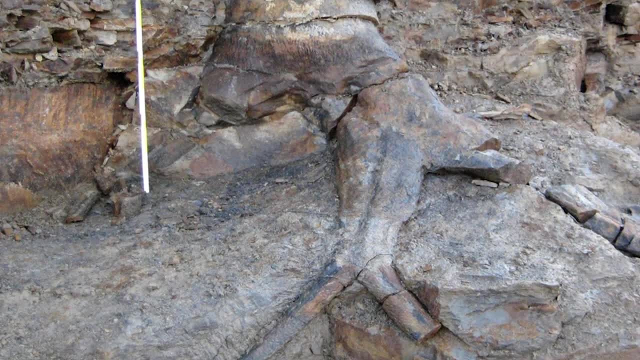 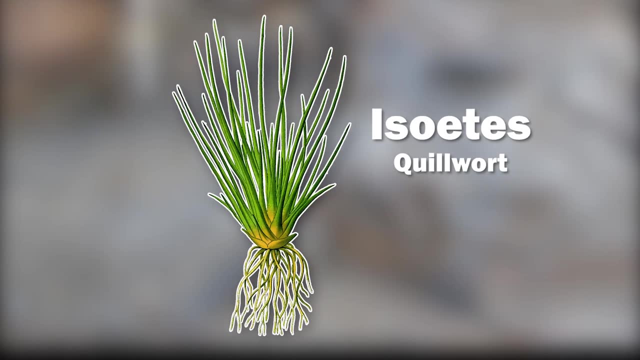 The root system of Sigillia, as Lepidodendron and overall Lepidophytes are closely related to the current Quilwort or Isoethes. Just like Lepidophytes, Quilwort has a root system characterized by the shape of the 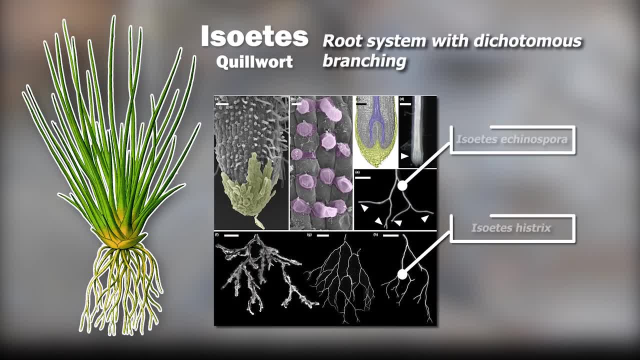 tree. Lepidodendron is the root system of Sigillia. Lepidodendron is the root system of Sigillia. Lepidophytes are characterized by its dichotomous branching and the presence of rhizomorphs. 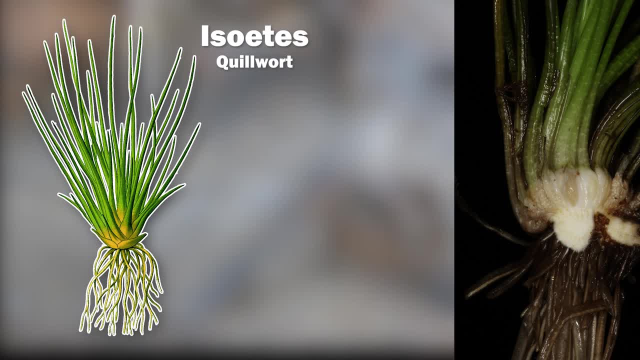 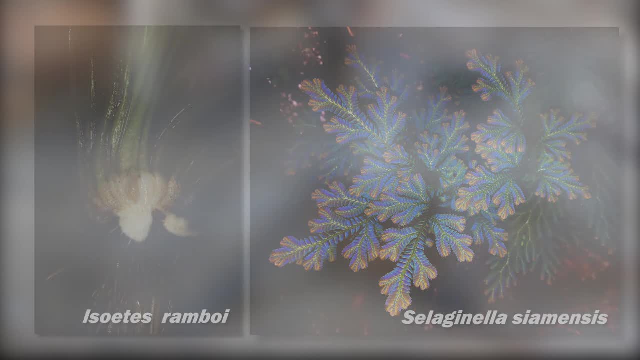 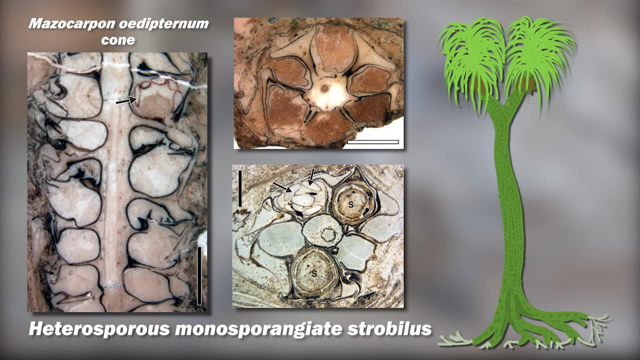 that is interpreted as an equivalent of the stigmian root system of Lepidophytes. Furthermore, as Quilwort and Sigillaginella, Sigillaria was an heterosporous lycophyte with monosporangiate reproductive organs resulting in cones called masocapones, which contained 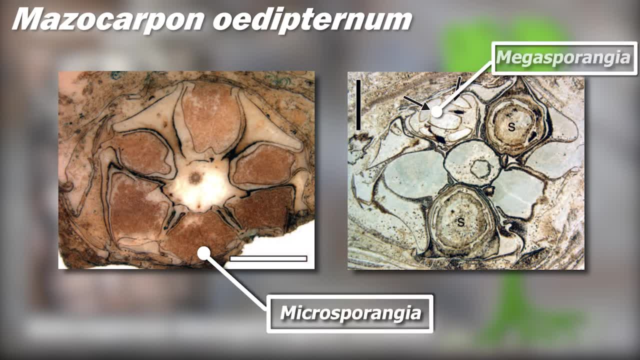 either microsporangia or the megasporangia. Lepidophytes are also known as Lepidophytes. Lepidophytes are also known as Lepidophytes. Lepidophytes are also known as Lepidophytes. 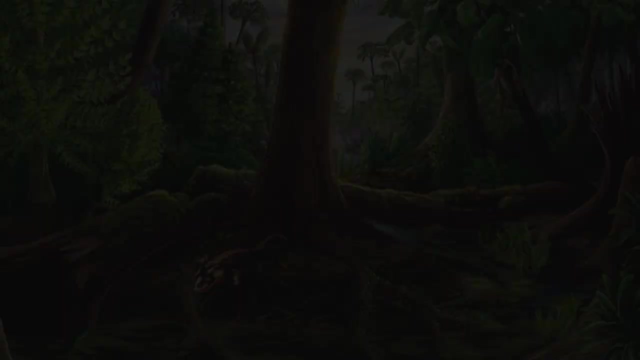 Lepidophytes are known as Lepidophytes. Lepidophytes are also known as Lepidophytes. Lepidophytes are also known as Lepidophytes. Lepidophytes are also known as Lepidophytes. 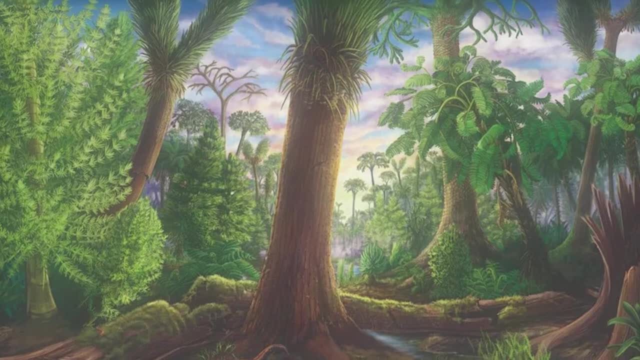 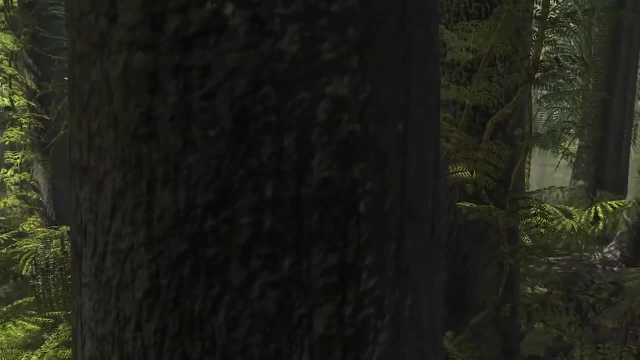 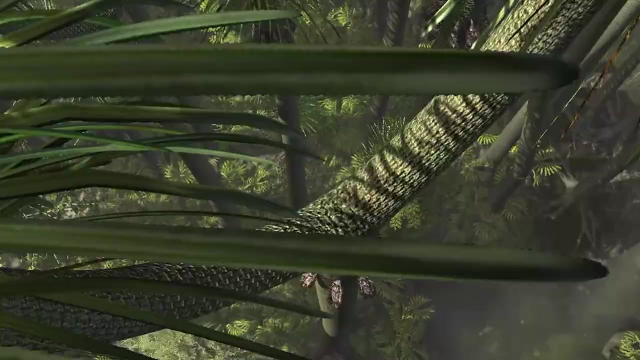 As a consequence, Sigillia and other Lepidophytes have a close kinship with Haisoetas, more related to each other than to Lycopsids. Sigillia could likely reach 30 meters tall and its crown resulting in dichotomous branching. 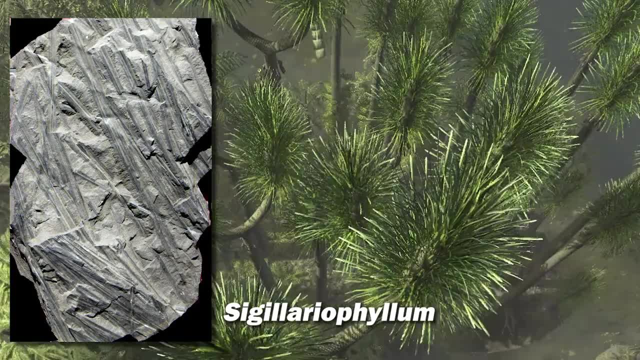 with two axes, sporting long and narrow microphyllox leaves. The Sigillarians are believed to haveивere to deserve a carrion-like germ, so that they can divide the maggots into denominations, depending how many organs aordum Golgiports has. 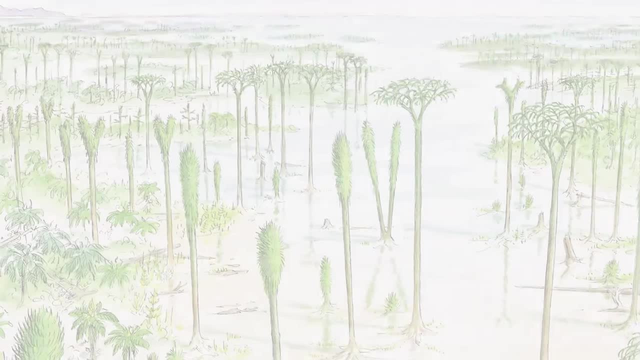 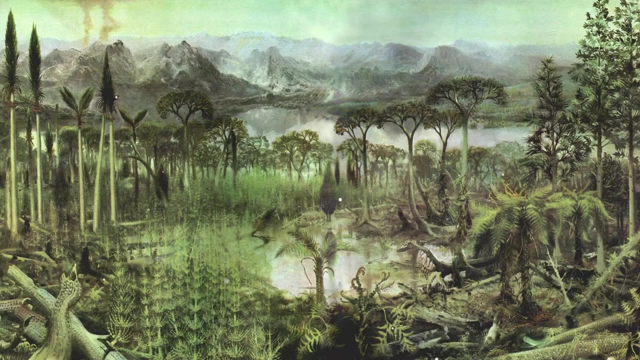 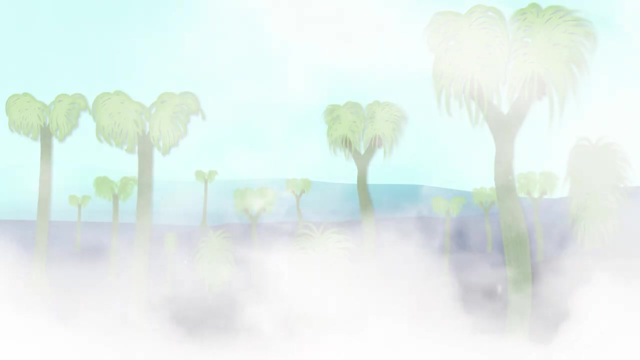 to have inhabited new swamps, environments that were slightly drier than those dominated by the other arborescent isotopes, just like lipidandron or synchysidandron. what a tropical rainforest of the late carboniferous and the early permian were sigillian, thrived, were the habitat. 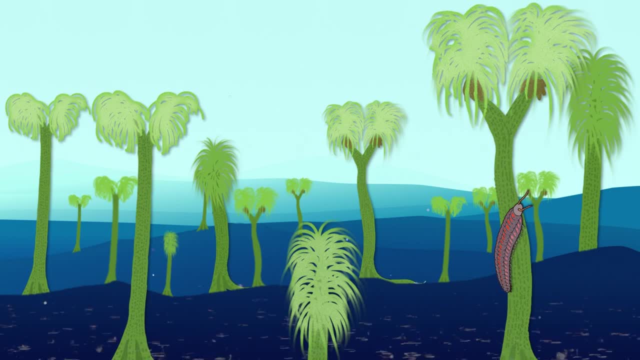 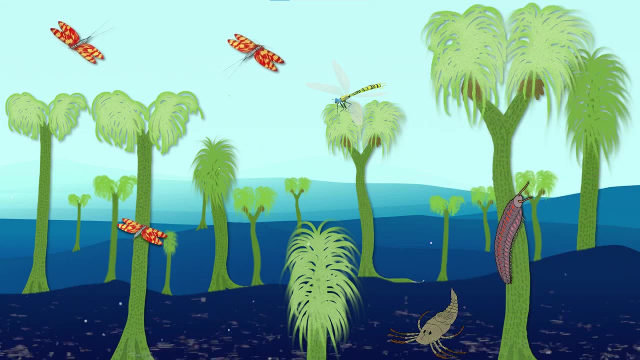 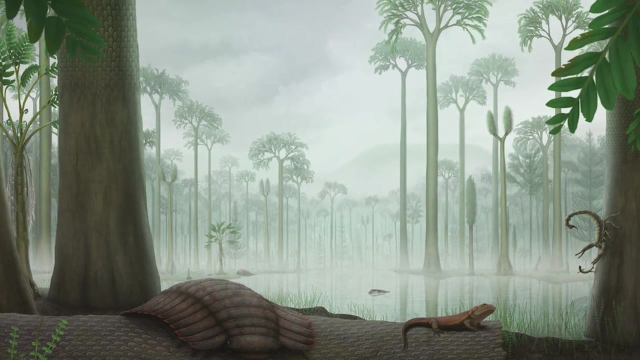 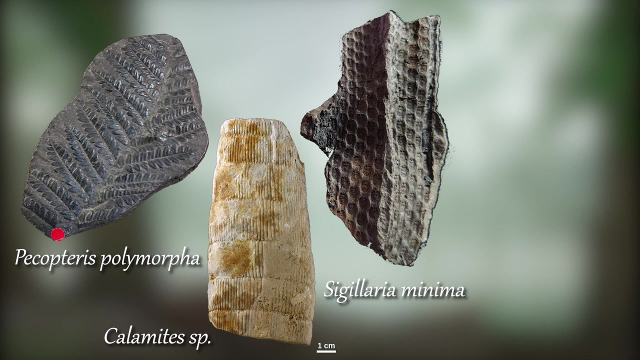 of numerous gigantic arthropods, species like the arthroplerids, meganura, paleodictyopterans and the freshwater steroneurina called megarachni. the rainforest was also an environment that presented a great diversity of ferns, lycophytes, giant oastale as calamites and the first seed,